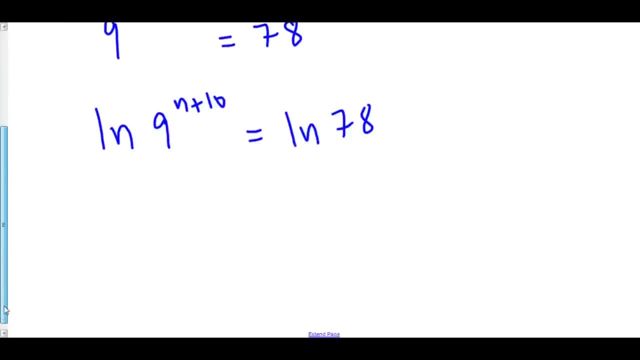 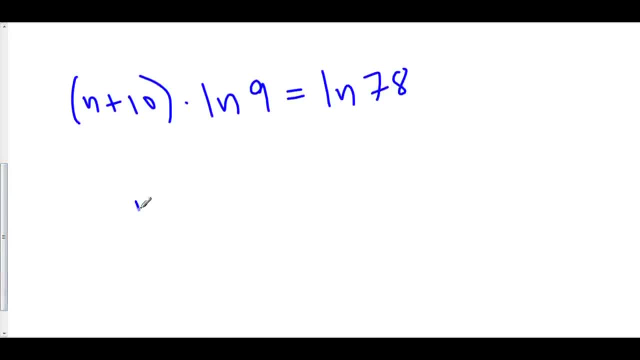 by the natural log of 9 and we get n plus 10 is equal to the natural log of 78 over the natural log of 9.. And finally, we can subtract 10 and we get n is equal to the natural log of 78. 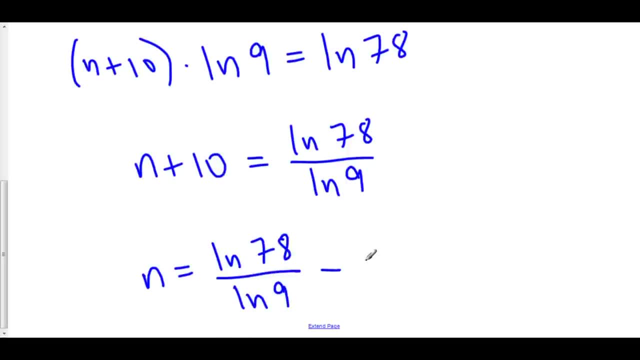 over the natural log of 9 minus 10.. And we can just leave it like this. actually, That is what n is equal to. Let's try another one: 5 times 6 to the 3m is equal to 20.. Well, first we want to get our 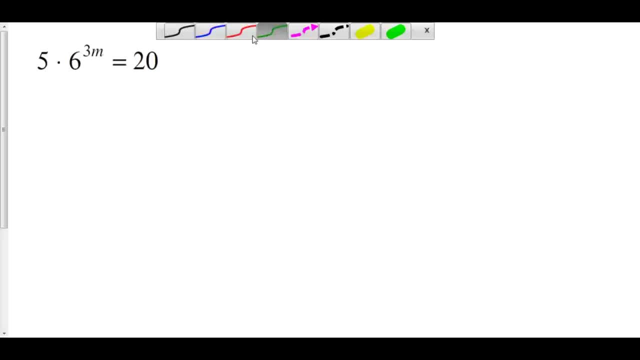 base and exponent on one side by itself. To do that, we'll divide by 5.. So we have 6 to the 3m is equal to 20.. So we have 6 to the 3m is equal to 20.. Well, first we want to get our base and exponent on one side by itself. To do that, we'll divide by 5.. So we have 6 to the 3m is equal to 20.. 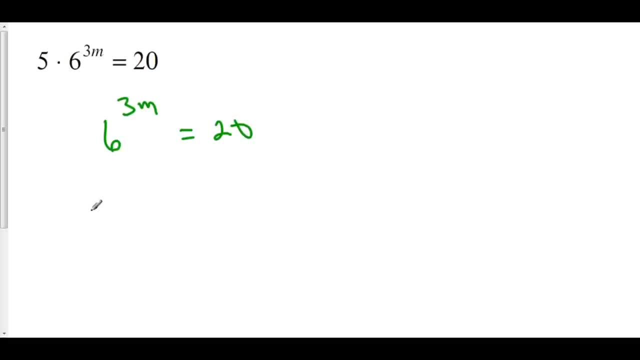 When we take the natural log of both sides, we get 3m times the natural log of 6, is equal to the natural log of 20.. That means that 3m is equal to the natural log of 20 over the natural log of 6.. And of course we can divide by 3.. And so m is equal to the natural log of 20 over 3 times the natural log of 6.. 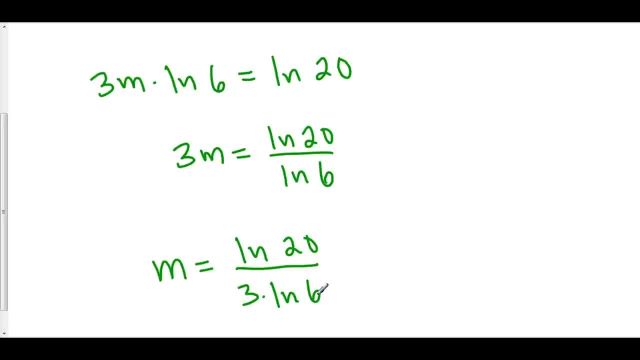 And we have solved the problem. Finally, 10 times e to the 10 minus 3m minus 8 equals 23.. Let's solve for m First. we'll add 8 to both sides, So we have 10 times e to the 10 minus 3m is equal to 31.. Divide both sides by 10.. So we have e to the 10 minus 3m is equal to 31..